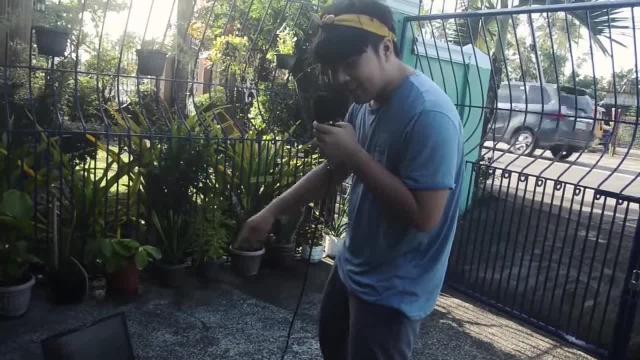 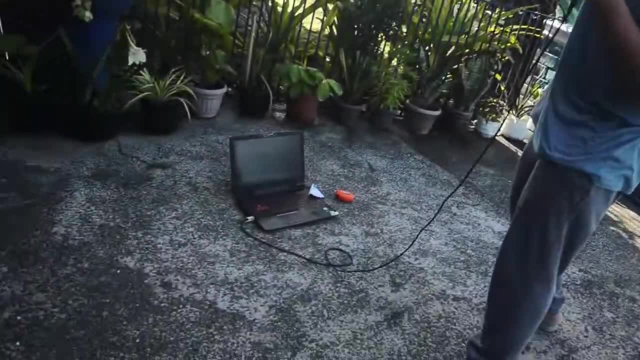 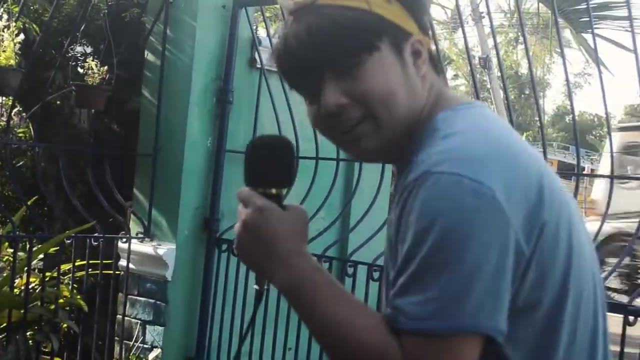 So the first thing we have to do is we have to use the measuring tape. to Shut up, We have to measure the base of the wall thingy, The tall structure to the place where I'm gonna use the clinometer. So to do that, we need this thing. 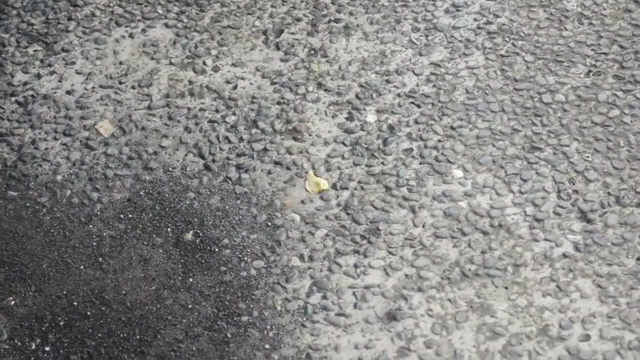 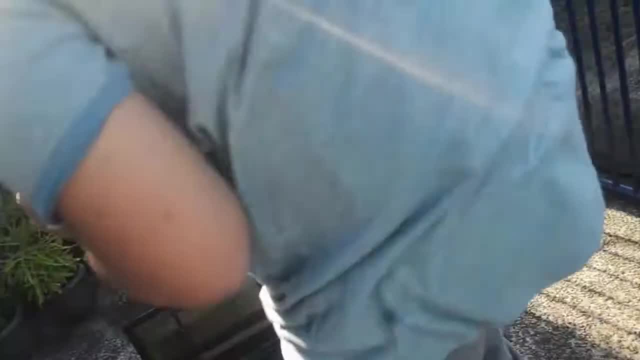 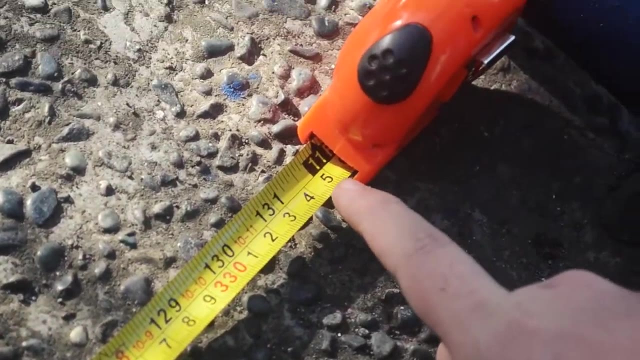 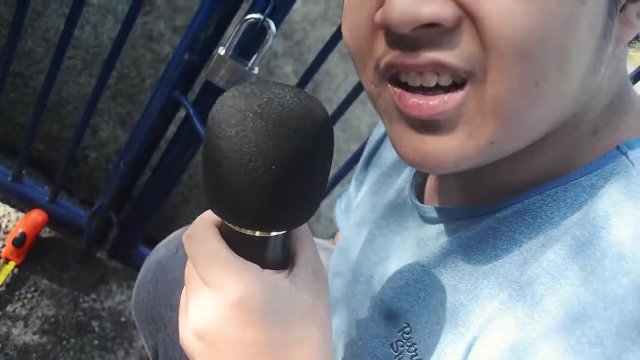 That is a fine reference. If you come closer, what does it say? Oh, where is it? 11 feet, You're wrong. Actually it's 335 inches. We do not use feet because we're not American. Wait, do Americans use inches of feet? 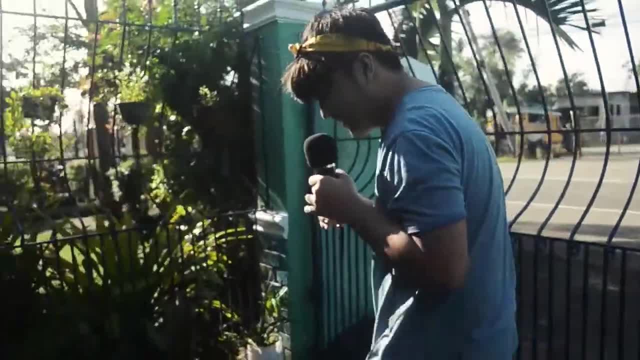 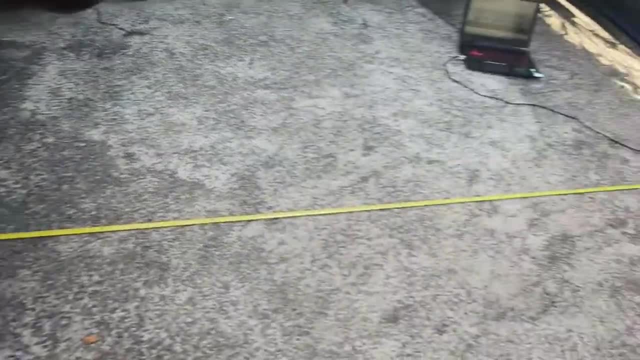 Of course you don't. You're the inferior sibling of the Ramos family. Now to use the clinometer: We know the base- I wanna die, The distance between the tall structure and where I'm gonna use the clinometer. Now I'm gonna use it. 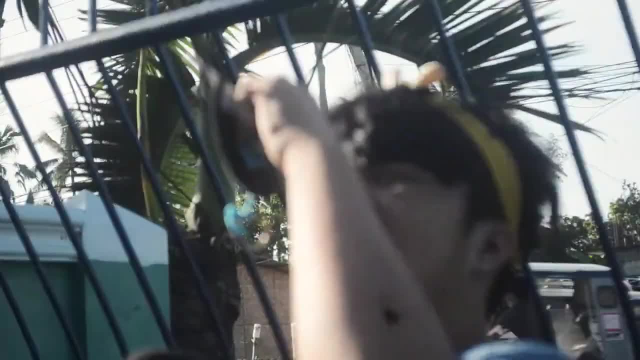 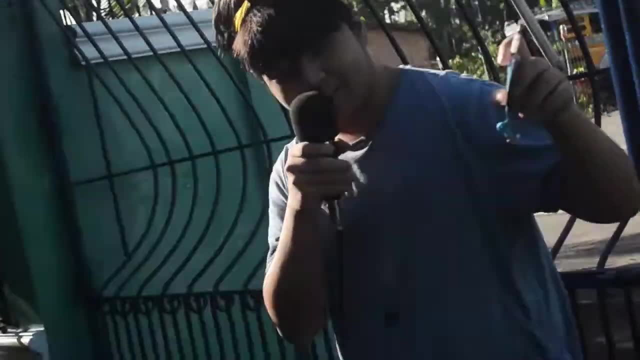 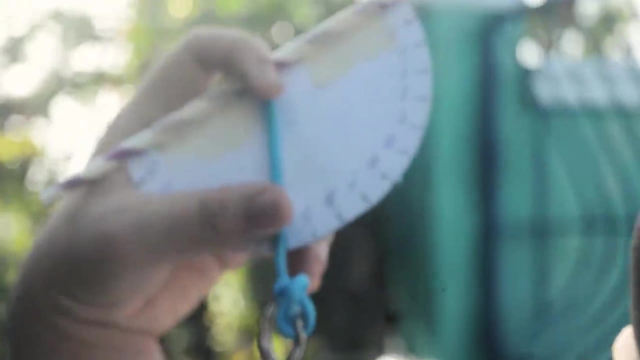 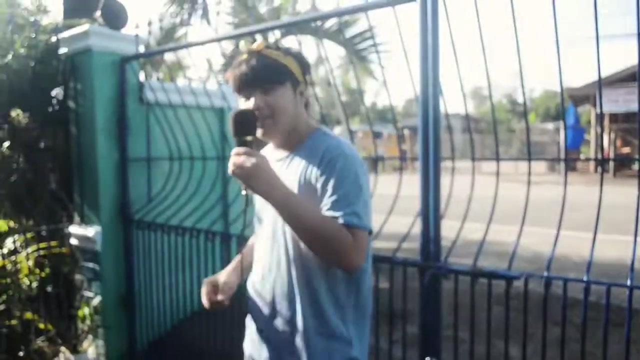 Oh, okay. So you see this. You see this masterpiece of clinometer. It says it's 20 degrees. 20 degrees, right Now, that's done. I don't need this clinometer. So now I go back to the room, suffer in calculating. 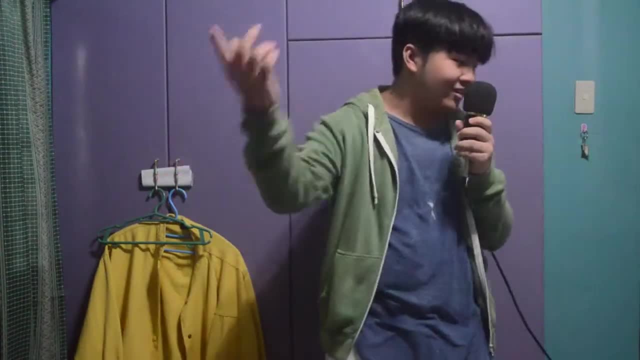 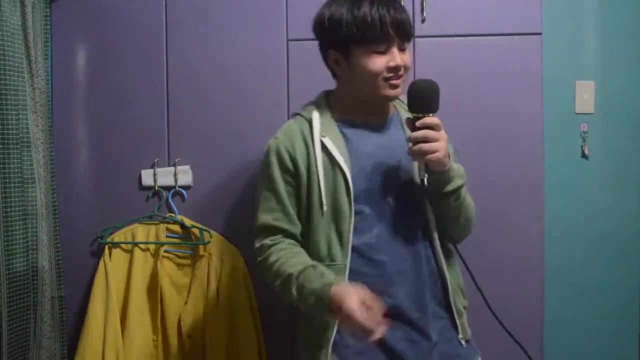 After all I did outside, I went inside and tried to look. Okay, I'm gonna try to measure the clinometer. now I'm gonna measure the height of the tall structure. Well, in the instructions that you gave me there's 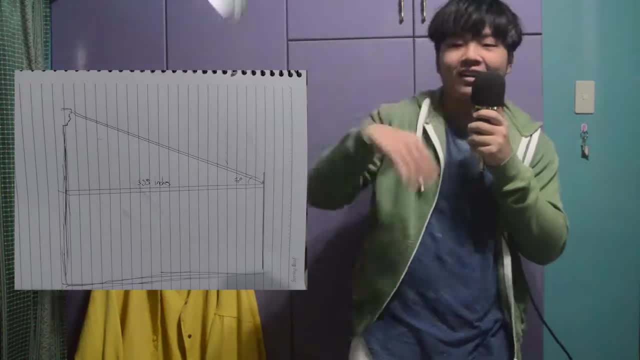 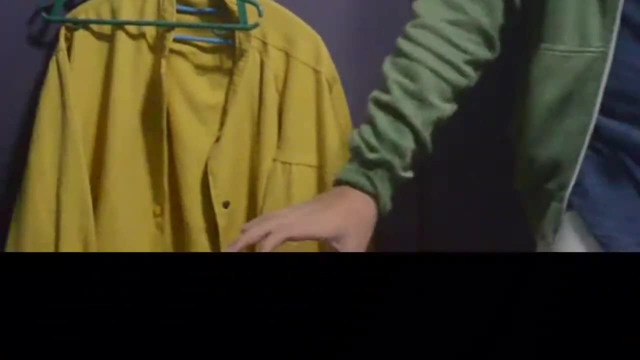 We have to sketch it right. You see this I'll put it in the video later, Since when I used the clinometer, of course it wasn't on the ground, so it's not really accurate. So what I measured actually was above my eye level. 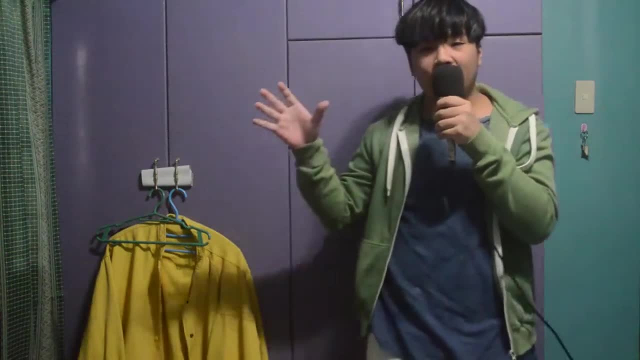 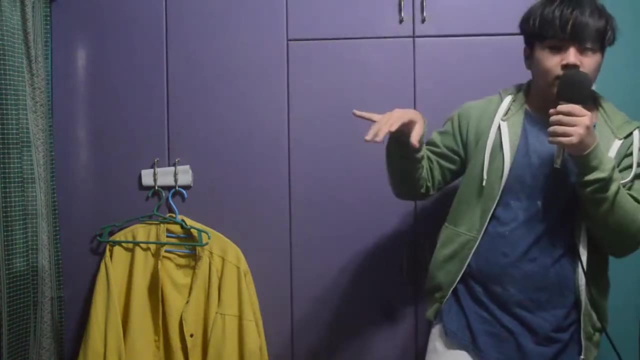 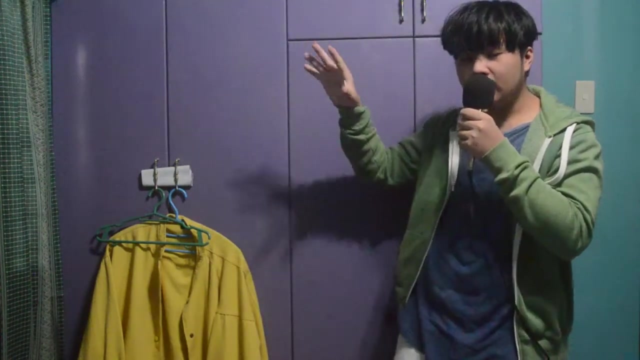 So it was basically my height. So first of all we're gonna measure the height of the tall structure- I'll just call it a ledge or a pillar. So we have to measure the height of the pillar above eye level. So basically the base formula is: tan x equals the distance between me and the pillar over the height of the pillar.